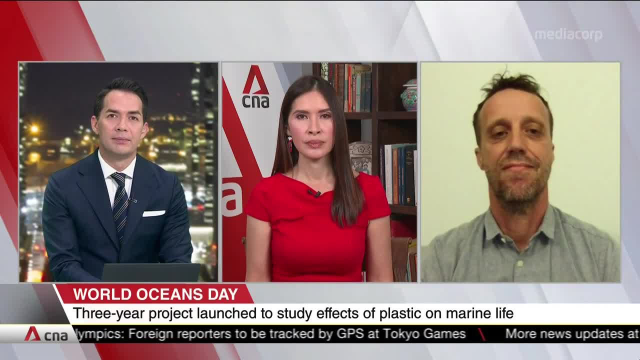 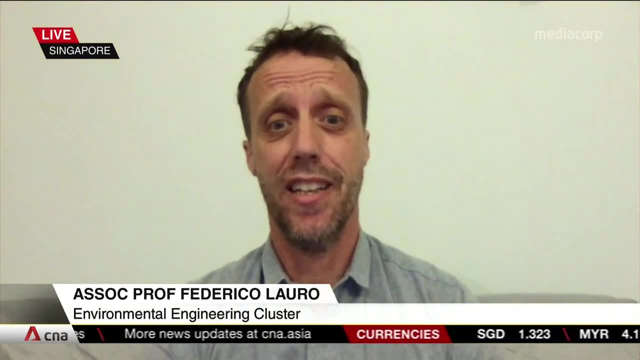 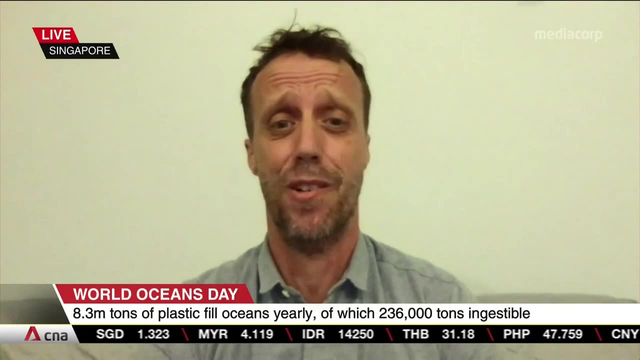 How do these plastics get into the ocean? Well, you know, plastic is an essential component of our everyday life In reality, and if you think about it, it's a fantastic material. We can use it to make pretty much everything, From toys to cutlery, to everything. 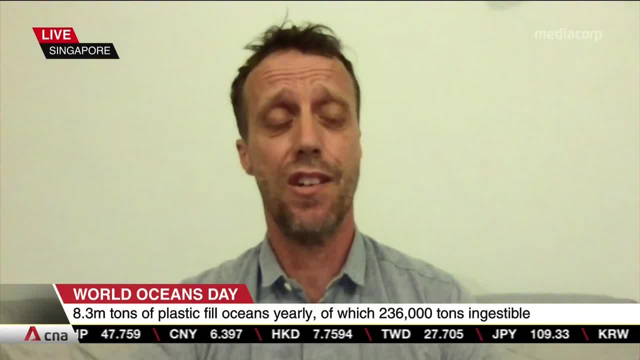 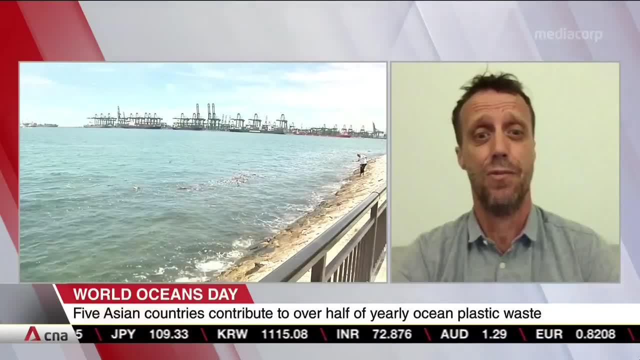 And it costs relatively little. Now the issue is not with the plastic that you reuse. I don't think we'll ever be able to get rid of plastic as a material. The issue is with the single-use plastic and the fact that people do not worry about recycling it. 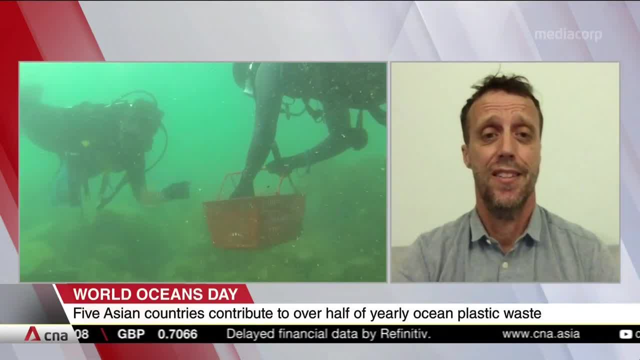 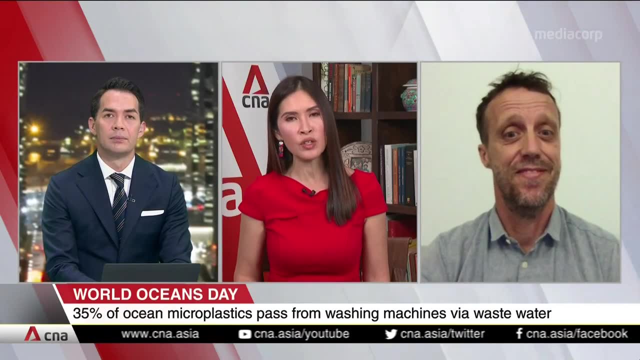 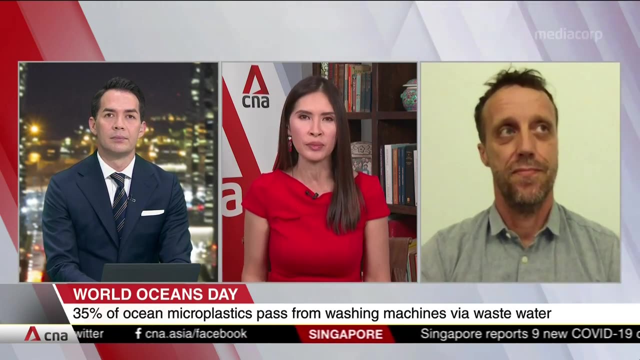 And that's the biggest problem, Professor Lauro, that's despite more ambitious efforts by governments and conservation groups as well. They've been trying hard to stop that plastic from getting into the ocean. So where is it all coming from? 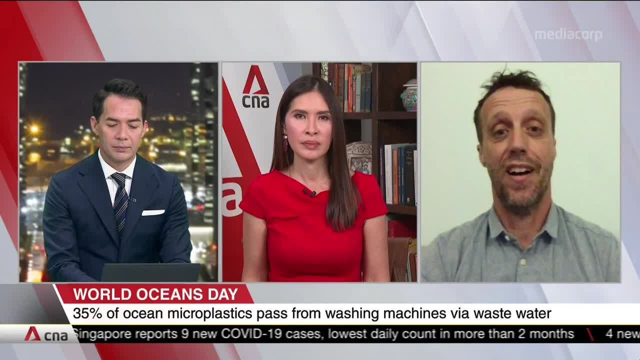 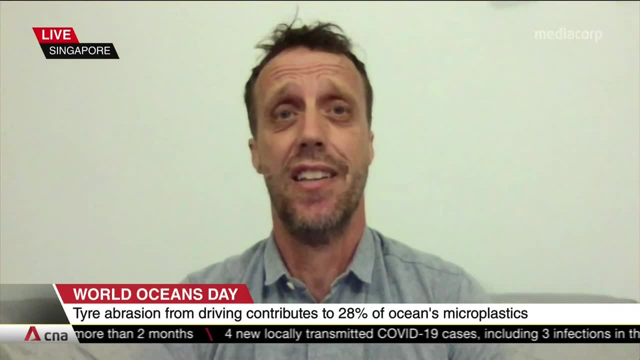 As I said, it comes from our normal everyday life. I mean, if you think about how many people go shopping every day and get a plastic bag, I get offered a plastic bag every time I buy the smallest thing from a candy Two. 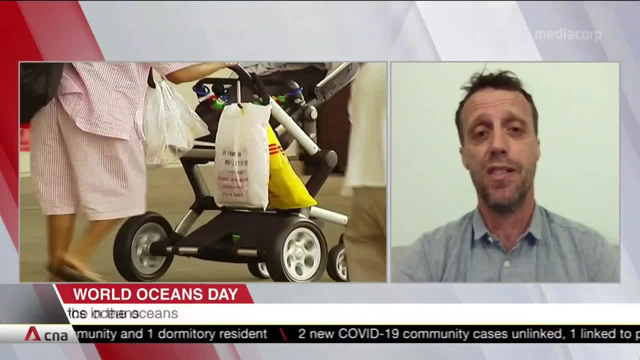 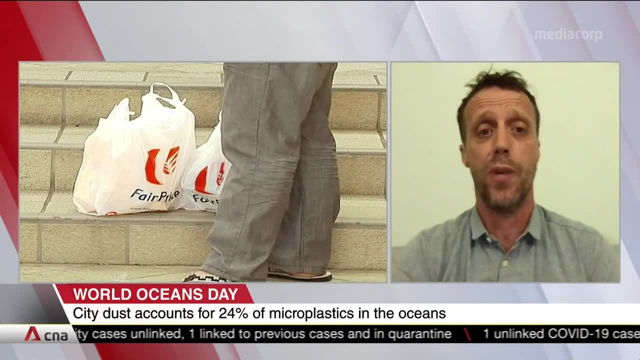 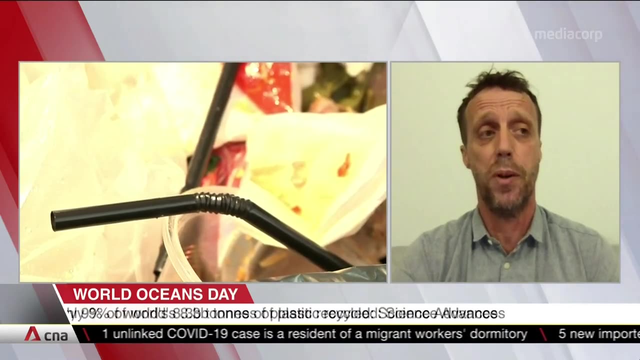 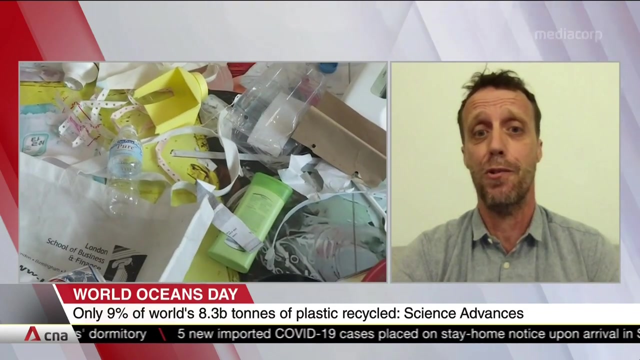 To anything, And so I think it's a responsibility of everyone to stop basically using single-use plastic And instead bring your own plastic bag to the market to do your shopping. I think that is an essential component, And it goes beyond that, of course, from bubble tea to single-use water bottles, to exactly all of that. 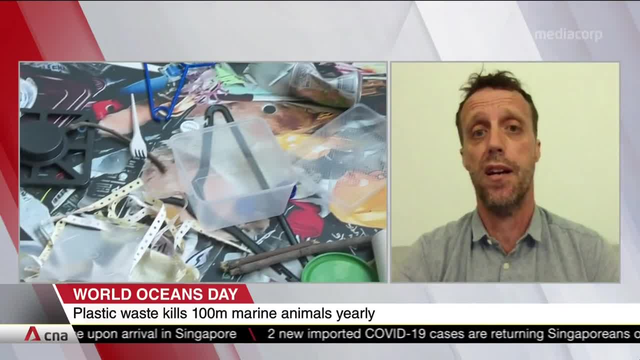 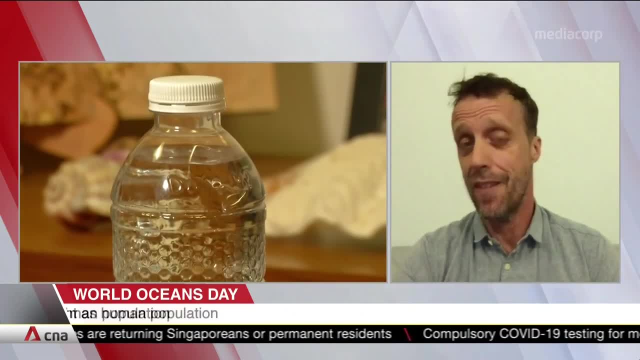 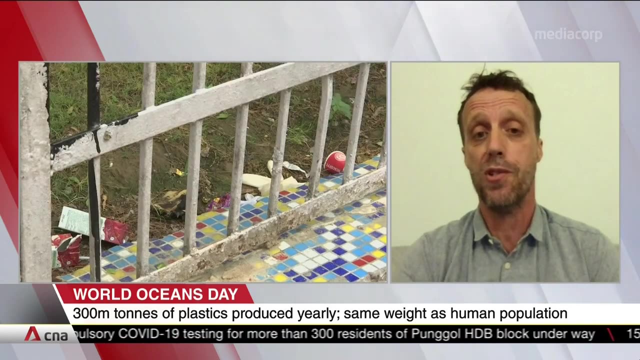 Those are, Those are the biggest issue. And then all of this ends up in eventually in a landfill, if we're lucky or more unlucky, in the water. Now I have to say that, in a way, COVID has amplified this effect, because we're taking away most of our food. 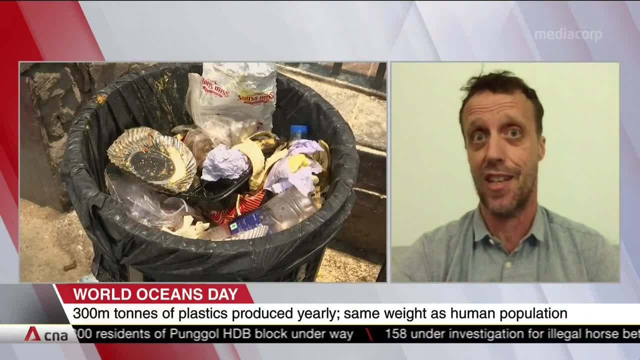 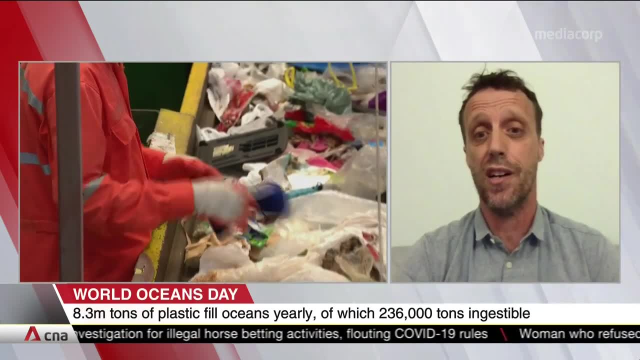 We're not able to eat on cutlery that just gets washed, And it's, I think, a responsibility of everyone to make sure that this actually goes: either recycling, Recycled or incinerated. Now we know that your team has just started the study. 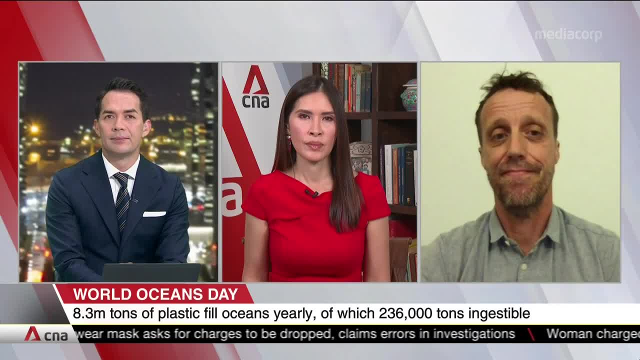 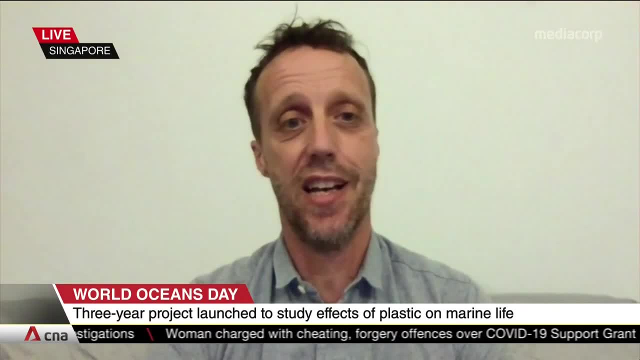 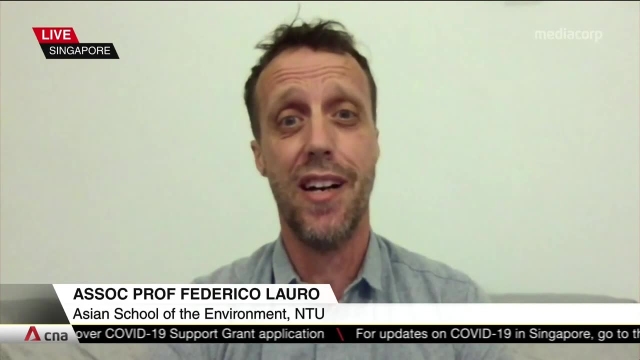 Any interesting finds so far? Well, a couple of them, I'd say. The first one is how much of the plastic is actually in very small sizes- And here we're talking invisible sizes at the micrometer level, Stuff that you would not even see if you didn't. 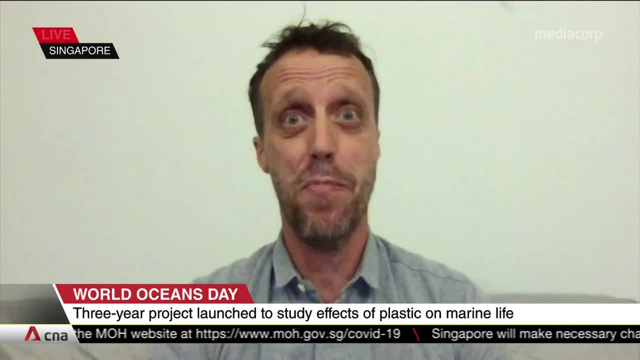 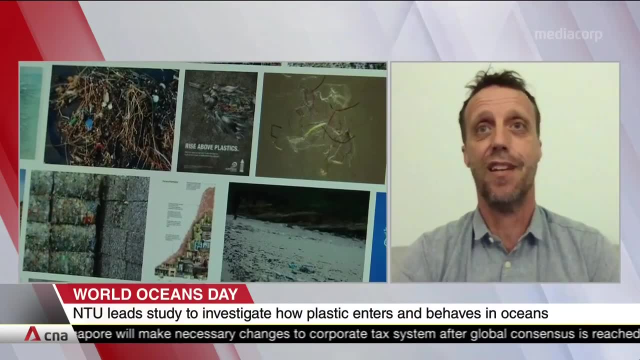 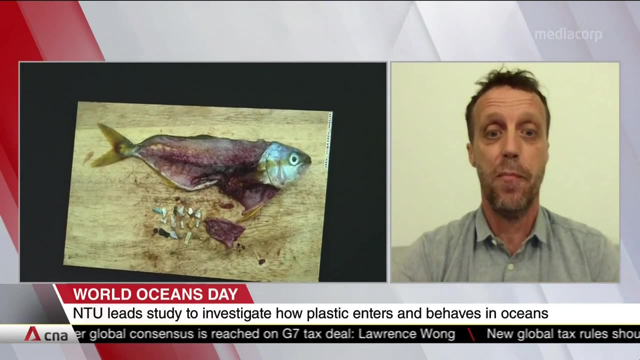 Even have a microscope. And the second thing is you can pick up consumer changes directly. by looking simply on the beaches, You start seeing, for example, disposable masks which contain a considerable amount of plastics And, of course, single-use containers for food takeout. 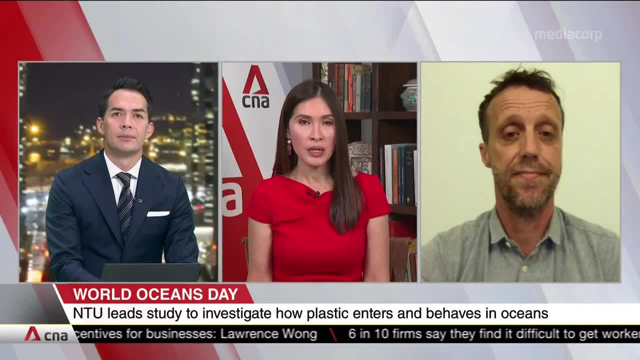 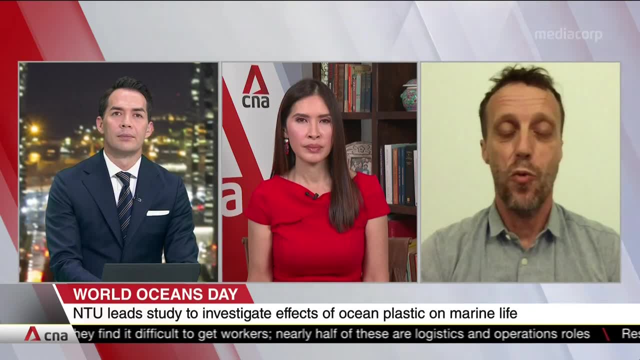 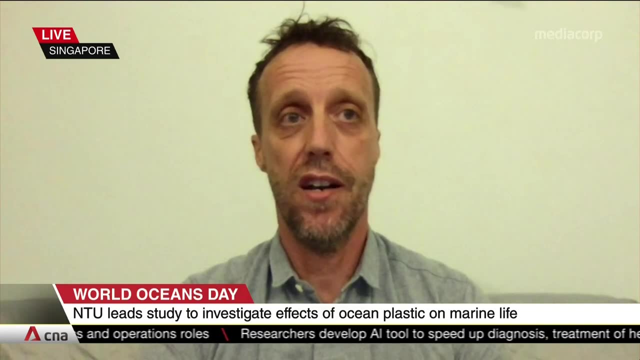 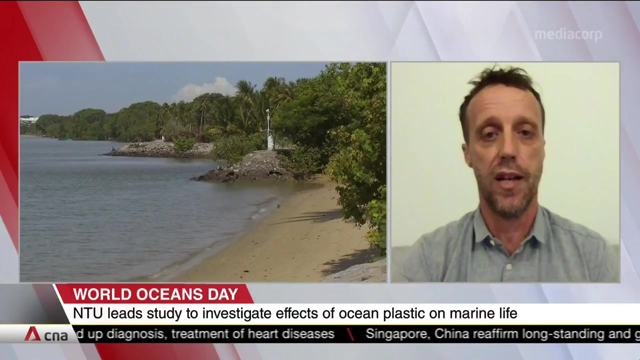 Professor Lauro, how devastating is this plastic problem For our oceans and the marine life in it? Well, the short answer is: we don't know yet, And that is there are not enough studies that have yet identified how problematic the different kinds of plastics can be to marine life. 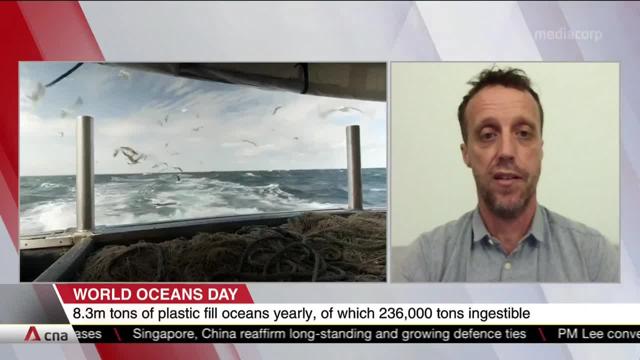 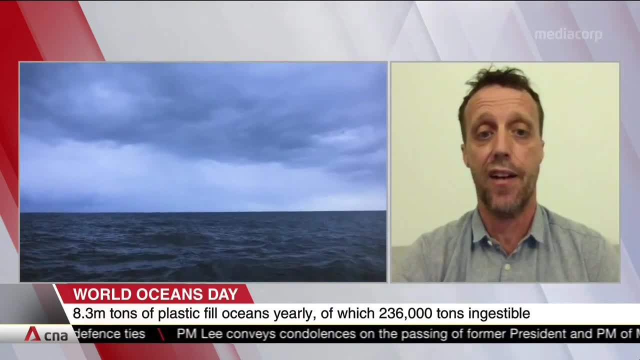 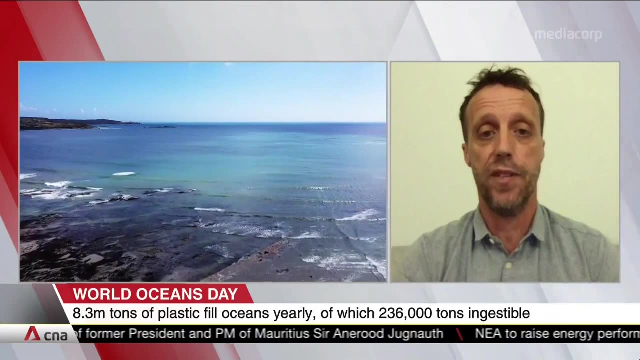 We know, of course, that macroplastics- the big plastic bags or cans, manholders or any of that- can strangle a lot of the bigger marine life. But what we don't know are the chemical effects of the smaller types of plastics that get ingested. 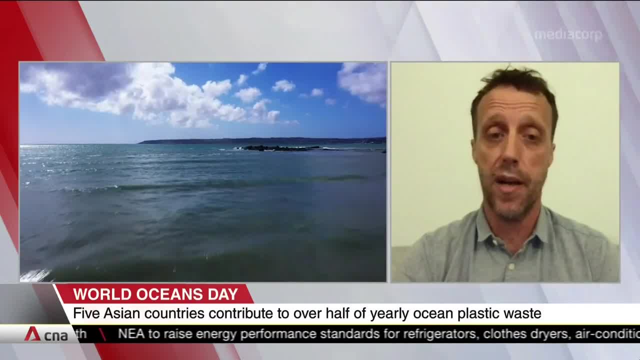 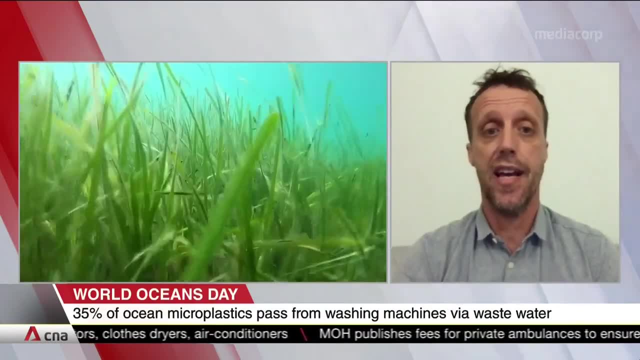 and then eventually gets accumulated through the food chain and might, and probably do, end up on our table every day. So that is the most problematic, I'd say, issue that we're still trying to tackle. I mean, in a way, we're 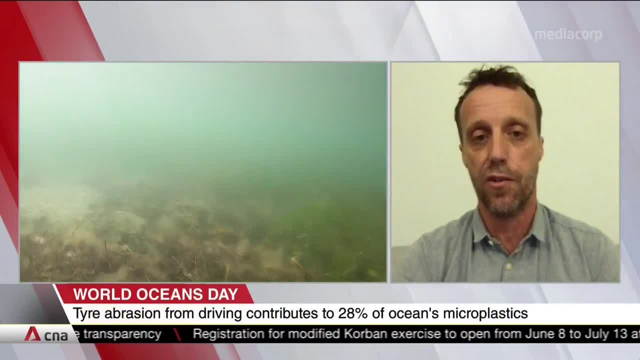 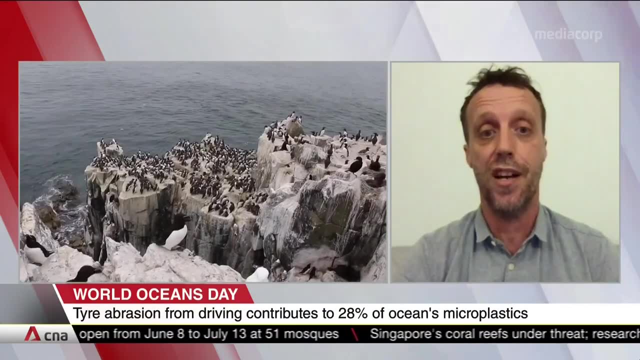 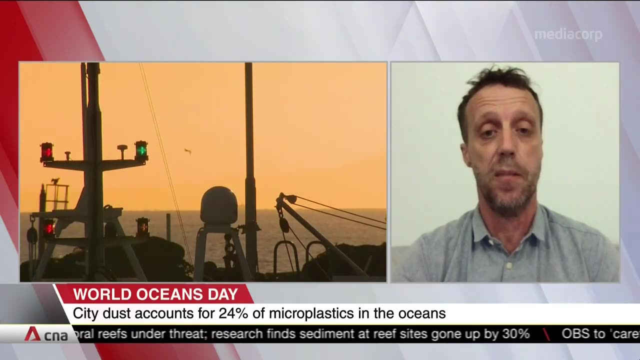 We're lucky that plastic is so difficult to degrade and so recalcitrant to degradation, But in a way that's also a benefit, because there are some studies that report that it just goes through the digestive tract of most animals without basically poisoning them with chemicals. 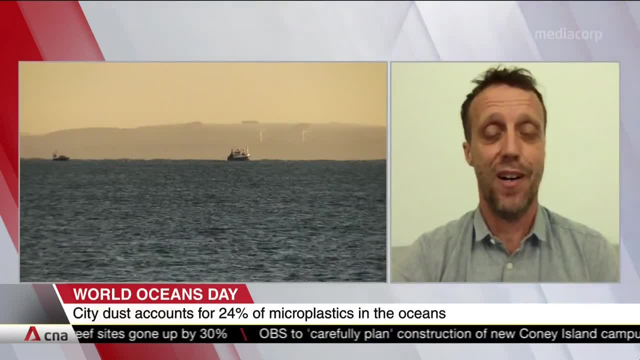 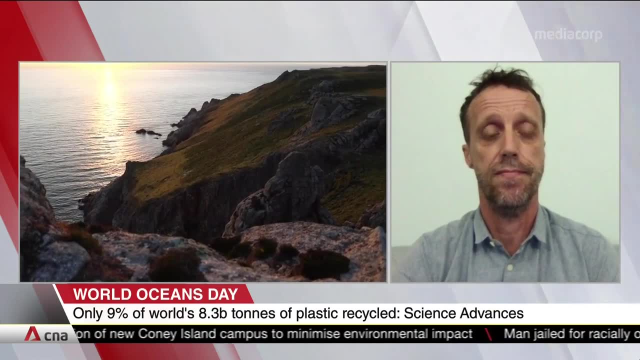 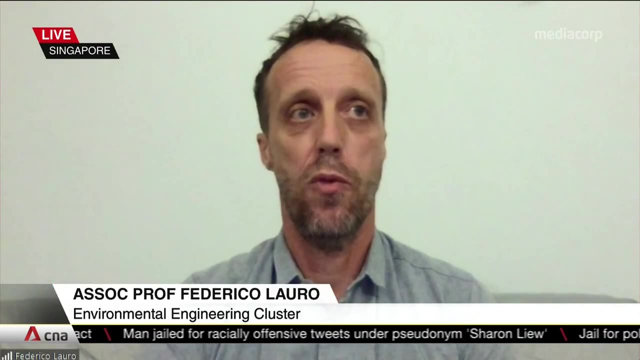 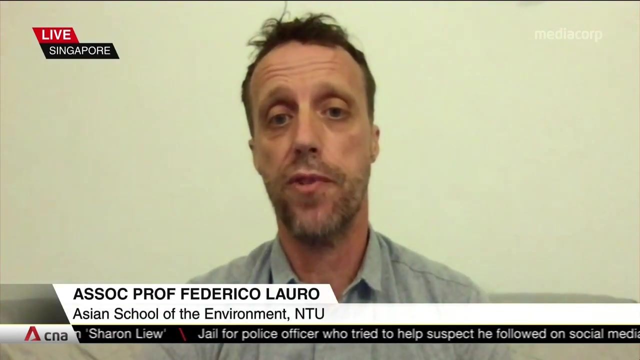 Now that doesn't say that we should be safe from preventing plastic from entering the oceans and to try to clean up the oceans in the first place. And how will the research be done? How will the results of your study be used? Well, first of all, we're getting the first long-term report and analysis of where the plastic is coming from in this region.